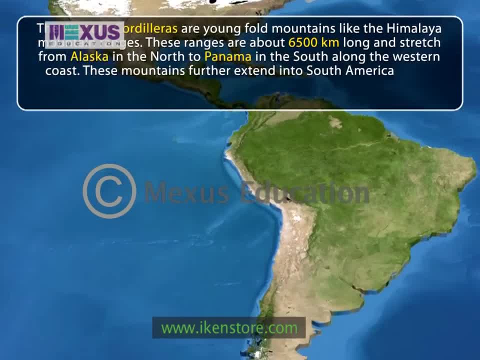 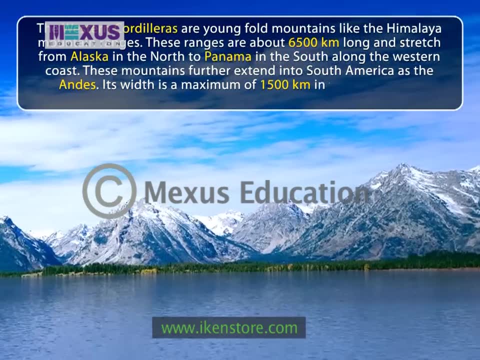 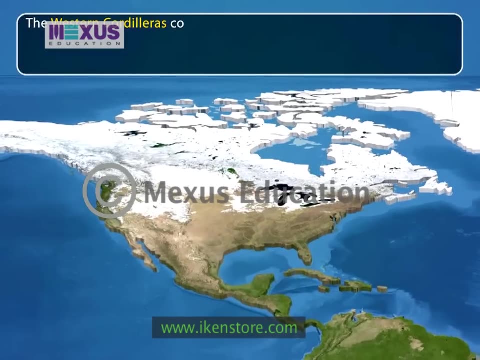 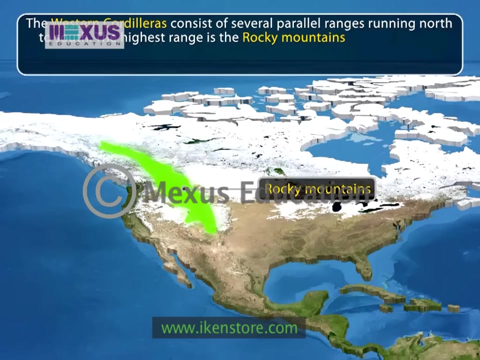 These mountains further extend into South America as the Andes. Its width is a maximum of 1,500 kilometers In the middle and decreases to the north and south. The Western Cordilleras consist of several parallel ranges running north to south. The highest range is the Rocky Mountains, which form the easternmost range. 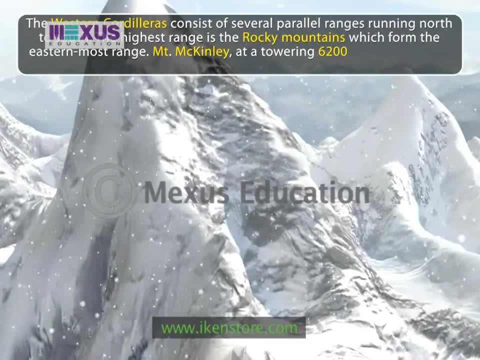 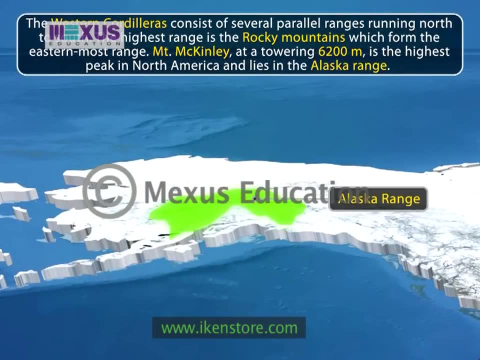 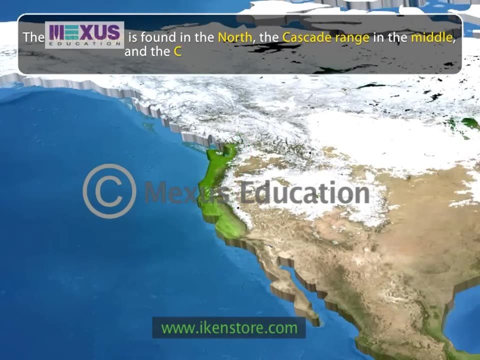 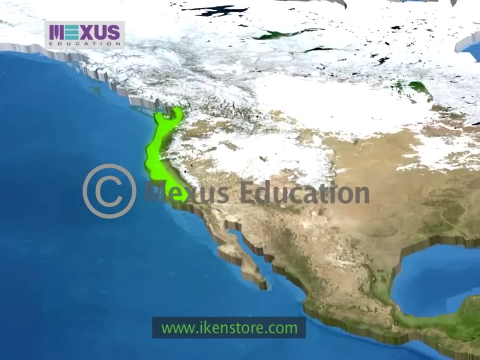 Mount McKinley, at a towering 6,200 meters, is the highest peak in North America. The highest peak in North America is the. The Alaska range is found in the north, the Cascade Range in the middle and the coastal range along the coast. The coastal range in particular rises steeply from the coast. 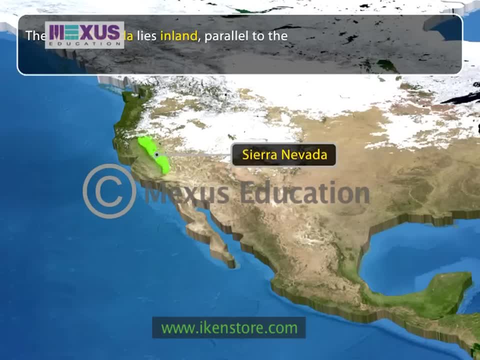 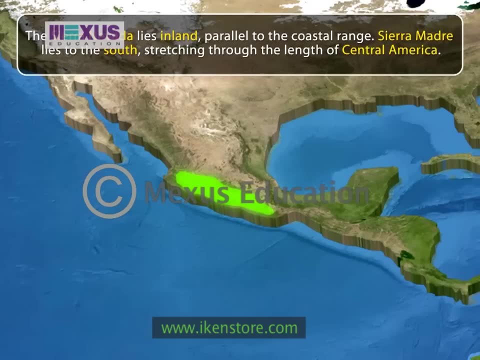 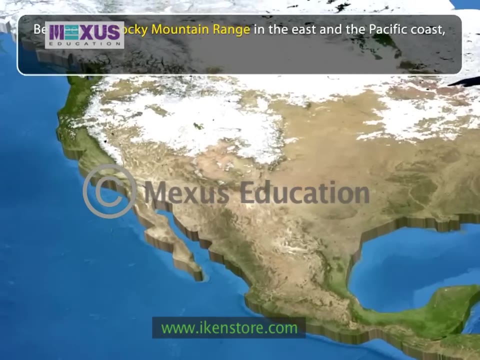 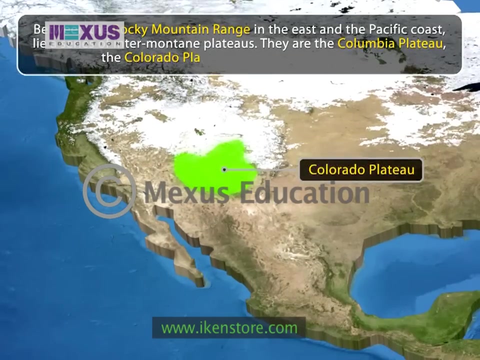 The Sierra Nevada lies inland parallel to the coastal range. Sierra Madre lies to the south, stretching through the length of Central America. Between the Rocky Mountain Range in the east and the Pacific coast lie a series of inter-mountain plateaus. They are the Columbia Plateau, the Colorado Plateau and the Mexican Plateau. 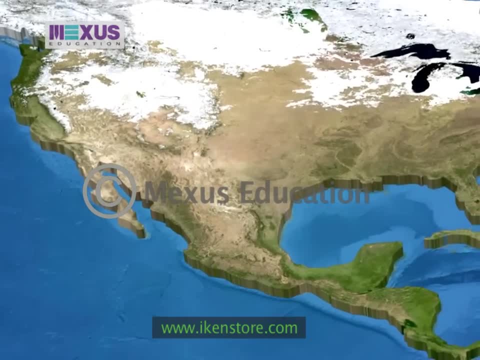 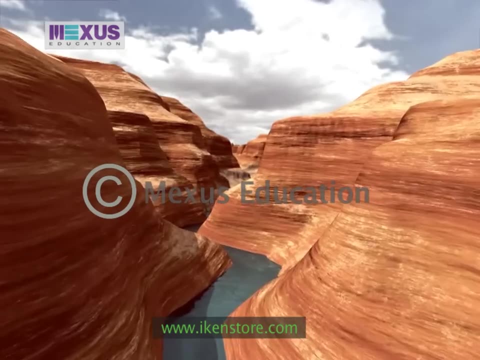 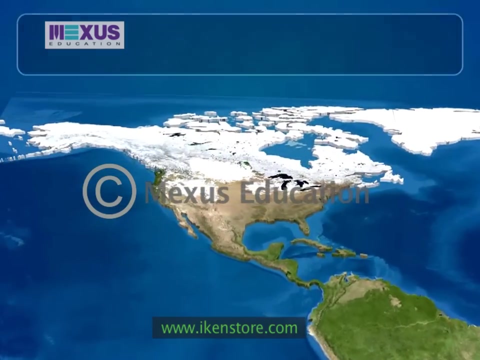 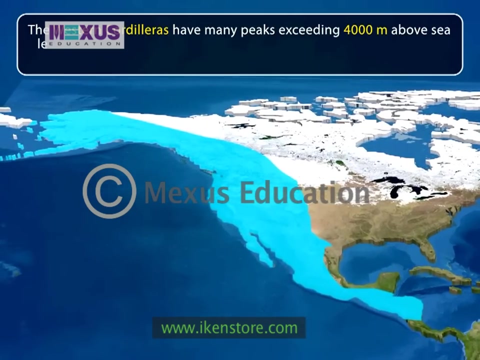 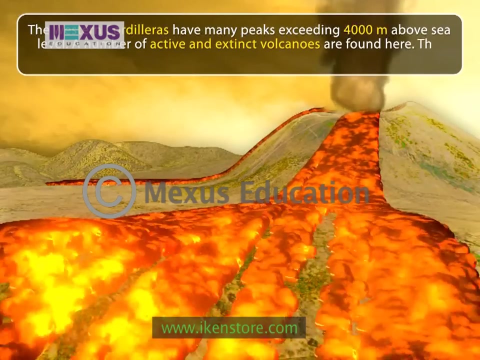 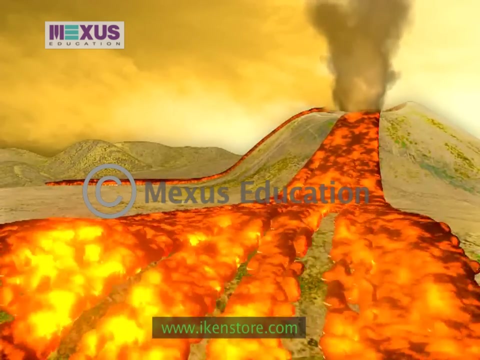 Many of these plateaus have been cut up by rivers. Some rivers, like the Colorado, have cut very deep gorges, known as the Grand Canyon, which is truly majestic. The best known for their vast coastline are the California Coast. The conversation between the two places is over. A number of active and extinct volcanoes are found here. The Western Cordilleras have many peaks exceeding 4,000 meters above sea level. A number of active and extinct volcanoes are found here. This is also a region known for earthquakes. Most of the rivers of North America have their sources in the Western Cordilleras. The South Caribbean has more than 90,000 water sources. The South Caribbean has a vast sea surface. Pink River Cay, a canyon in the north, is one of the most gripping waters in the US. 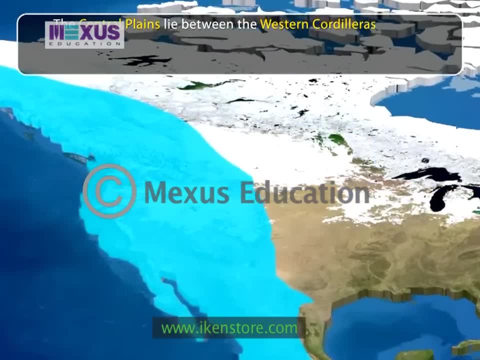 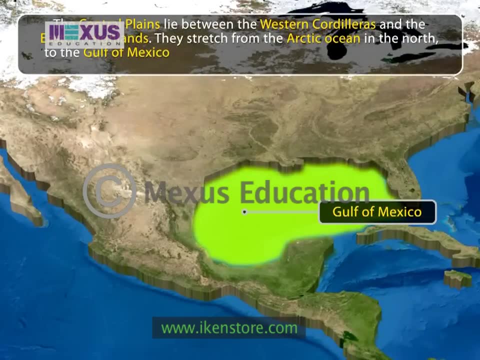 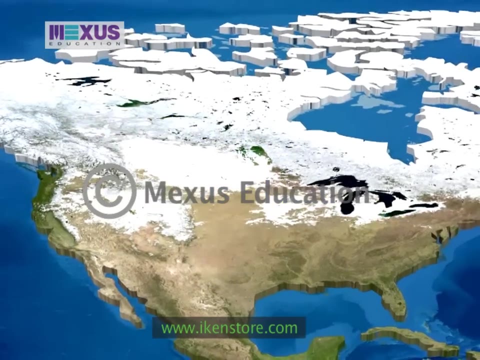 The central plains lie between the western cordilleras and the eastern highlands. They stretch from the Arctic Ocean in the north to the Gulf of Mexico in the south. These plains are also known as the Great Plains. The northern part, near the Hudson Bay, is known as the Canadian Shield. 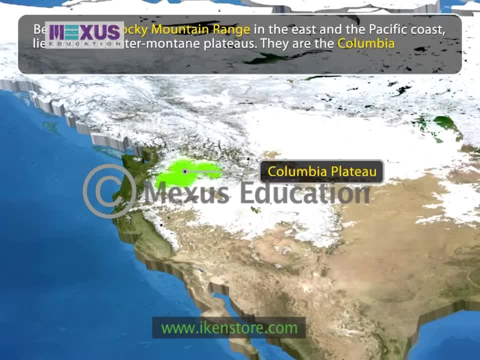 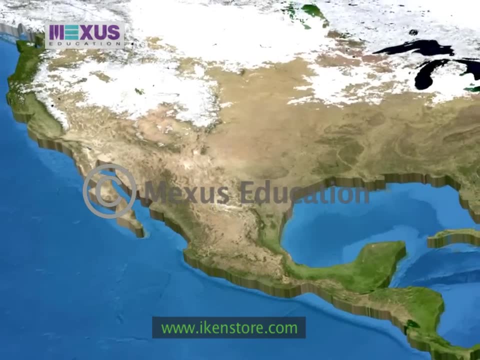 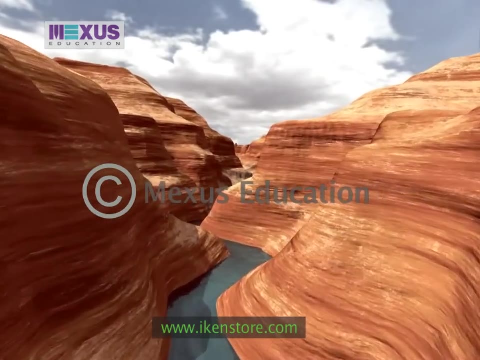 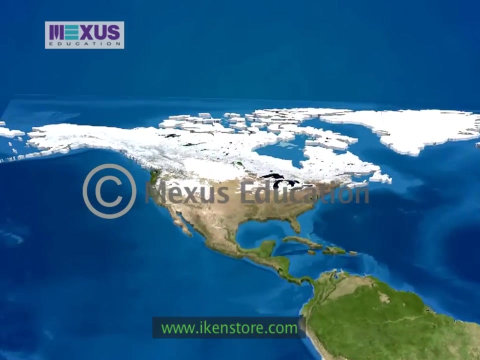 plateaus. They are the Columbia Plateau, the Colorado Plateau and the Mexican Plateau. Many of these plateaus have been cut up by rivers. Some rivers, like the Colorado, have cut very deep gorges, known as the Grand Canyon, which is truly majestic. 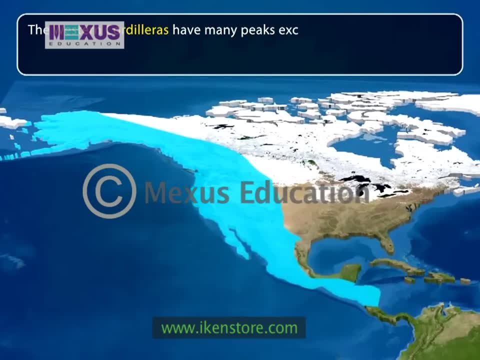 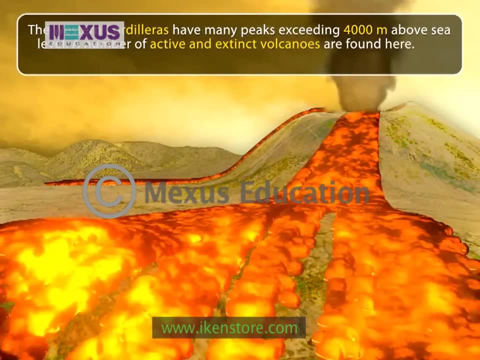 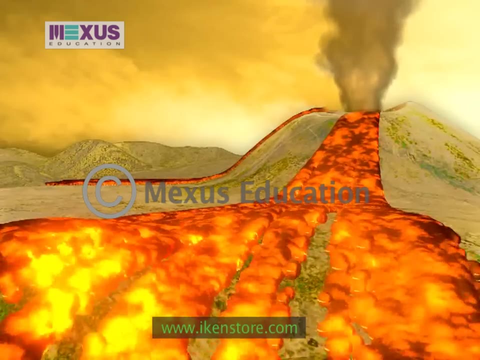 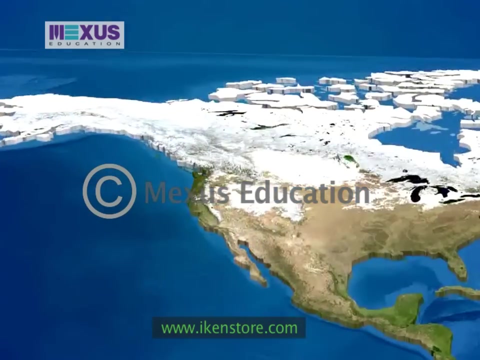 The Western Cordilleras have many peaks exceeding 4,000 meters above sea level. A number of active and extinct volcanoes are found here. This is also a region known for earthquakes. Most of the rivers of North America have their sources in the Western Cordilleras. 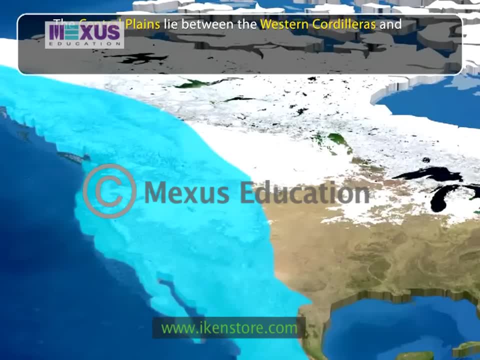 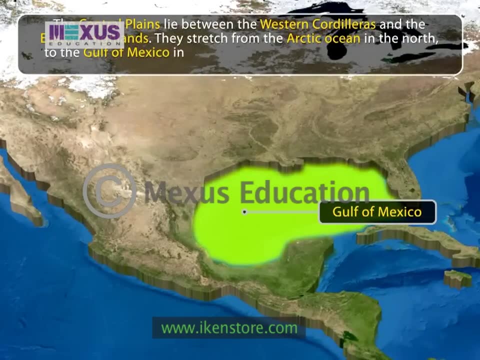 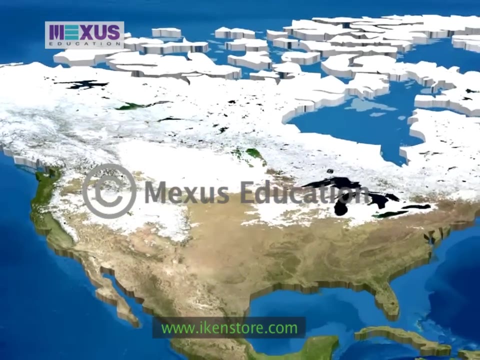 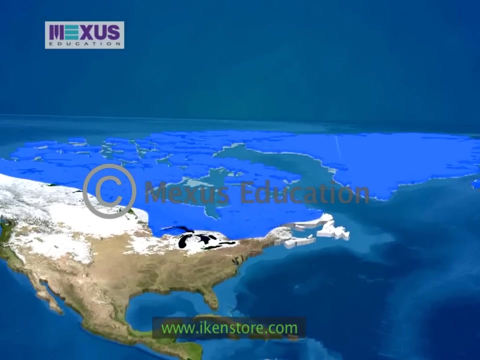 The Central Plains lie between the Western Cordilleras and the Eastern Highlands. They stretch from the Arctic Ocean in the north to the Gulf of Mexico in the south. These plains are also known as the Great Plains. The Northern part, near the Hudson Bay, is known as the Canadian Shield. It is made up of some 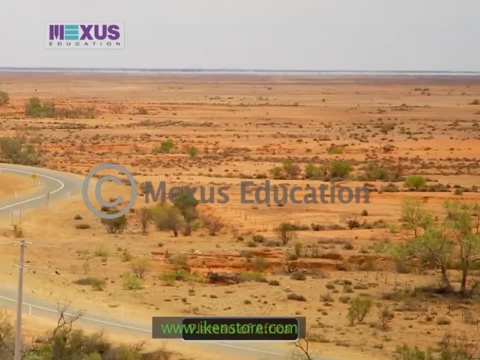 of the oldest rocks in the world. like the Plateau of Africa and the Deccan Plateau of India, The Canadian Shield is a large, very large-sized rock. It is the largest rock in the world. The Canadian Shield is the largest rock in the world. The Canadian Shield is the largest rock in the world. 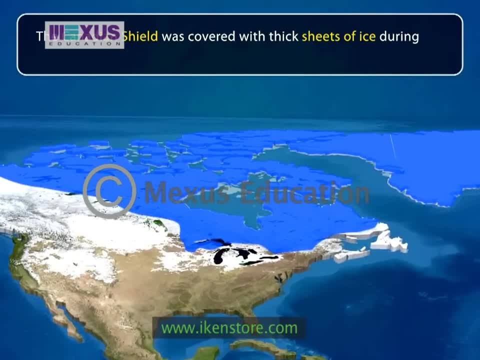 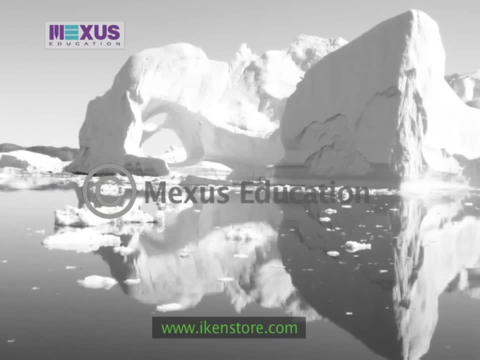 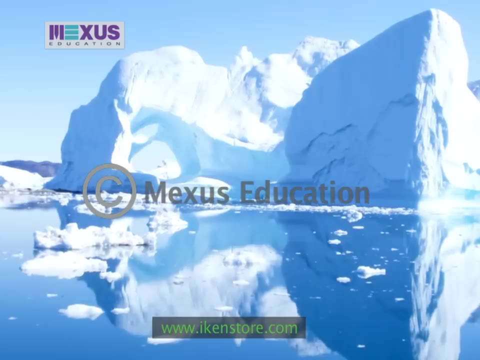 The Canadian Shield was covered with thick sheets of ice during the Ice Age about 18,000 years ago. Glaciers scooped out great hollows in the land as they slowly moved along. This resulted in the formation of thousands of depressions. 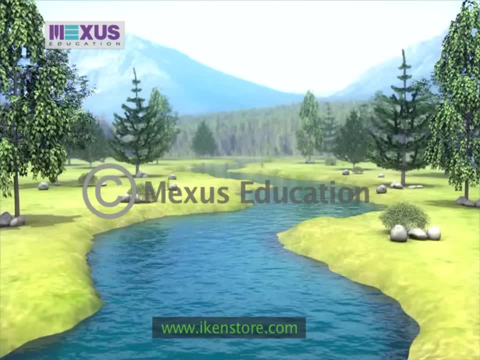 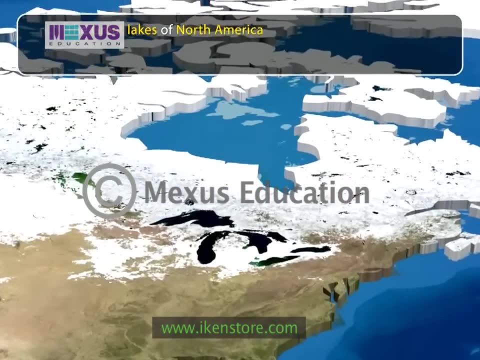 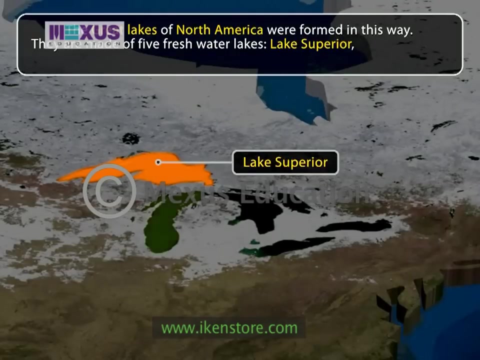 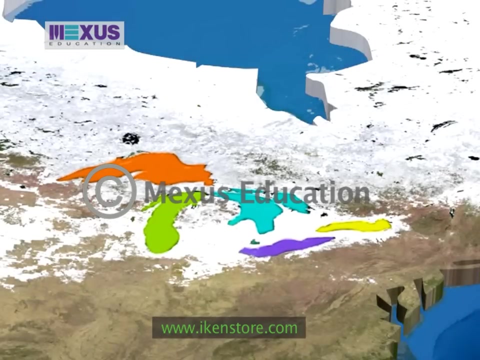 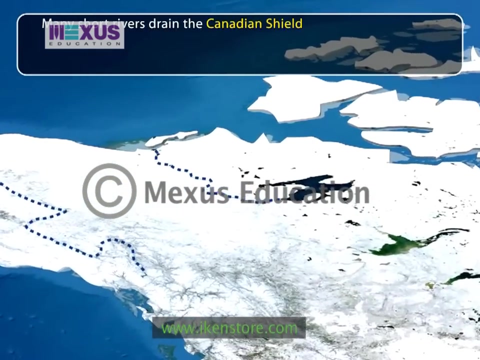 When the glaciers melted, water filled these depressions, forming lakes. The Great Lakes of North America were formed in this way. They are made of five freshwater lakes: Lake Superior, Lake Michigan, Lake Huron, Lake Erie and Lake Ontario. Many short rivers drain the Canadian Shield and enter the Hudson Bay. 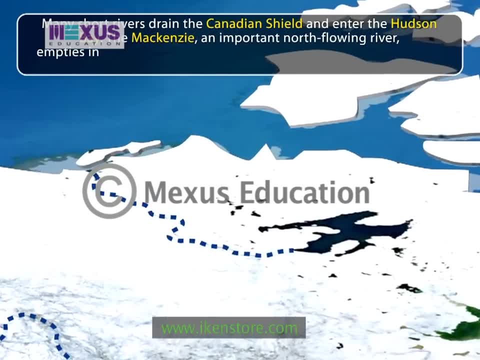 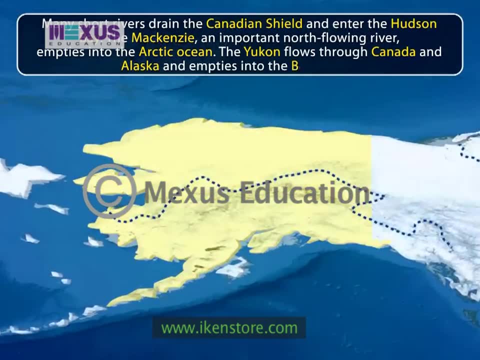 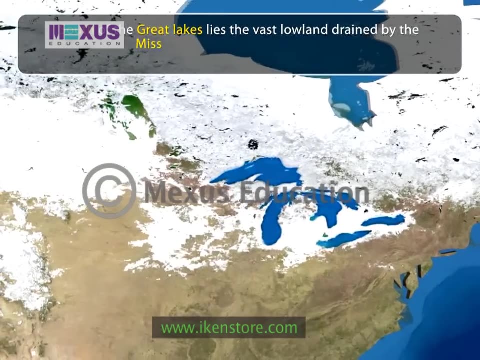 An important north flowing river empties into the Arctic Ocean. The Yukon, flows through Canada and Alaska and empties into the Bering Sea. South of the Great Lakes lies the vast lowland drained by the Mississippi River and its tributaries. 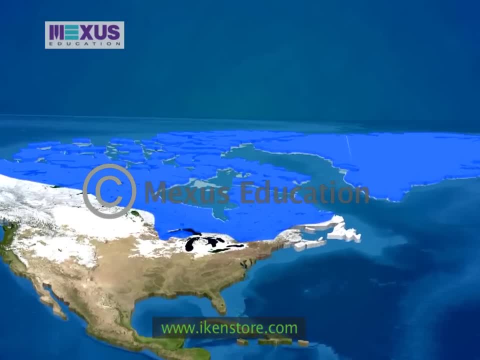 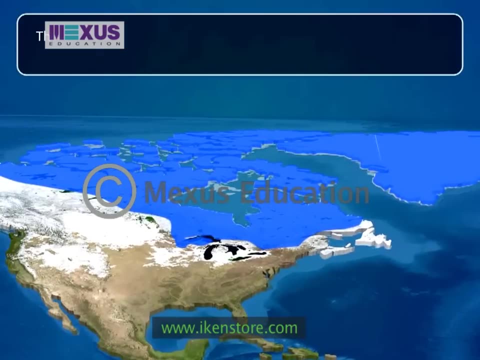 It is made up of some of the oldest rocks in the world, like the Plateau of Africa and the Deccan Plateau of India. The Canadian Shield was covered with thick sheets of ice during the Ice Age about 18,000 years ago. 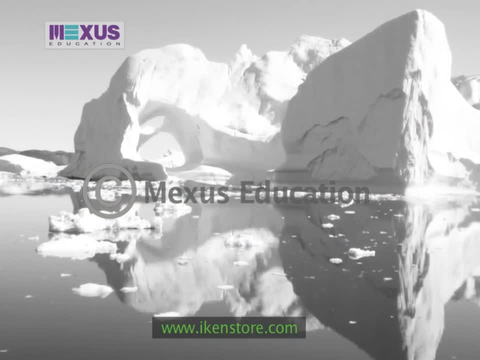 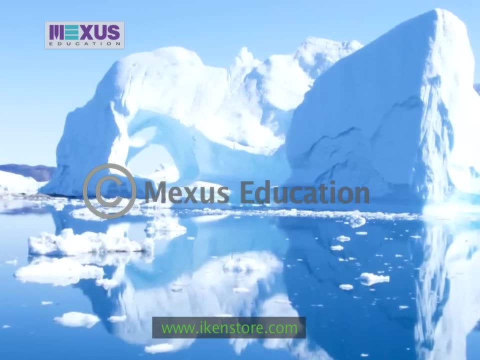 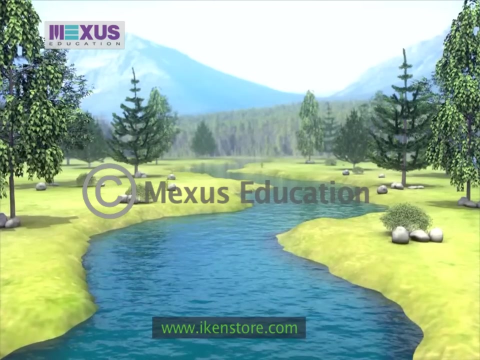 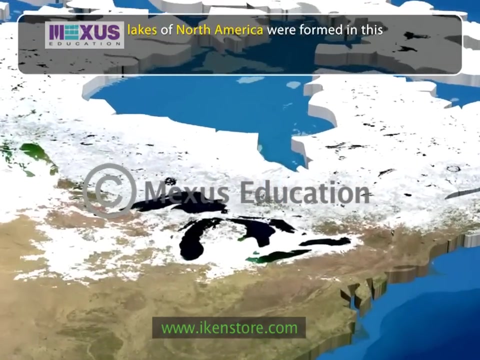 Glaciers scooped out great hollows in the land as they slowly moved along. This resulted in the formation of thousands of depressions. When the glaciers melted, water flowed and filled these depressions, forming lakes. The Great Lakes of North America were formed in this way. 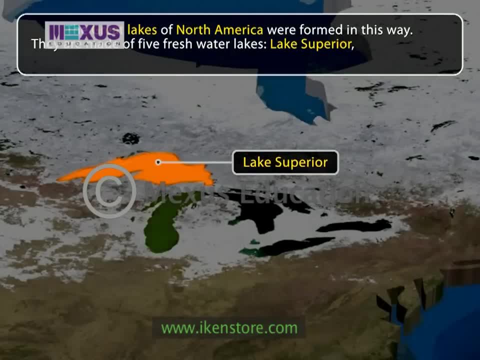 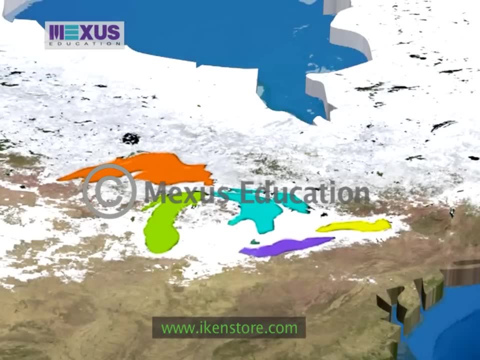 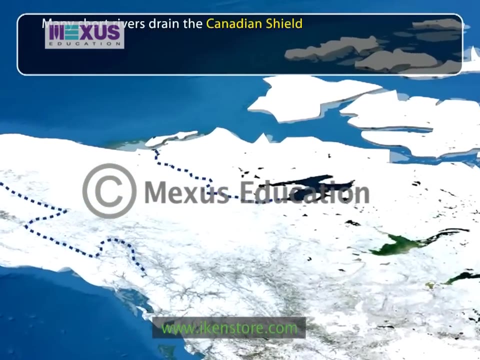 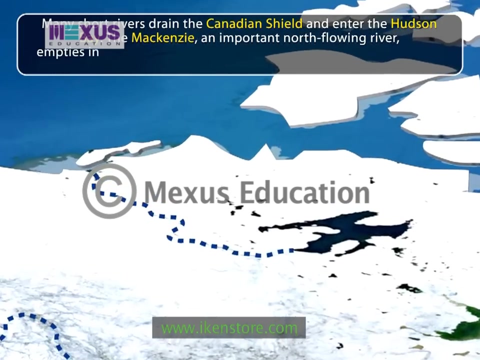 They are made of five freshwater lakes: Lake Superior, Lake Michigan, Lake Huron, Lake Erie and Lake Ontario. Many short rivers drain the Canadian Shield and enter the Hudson Bay. The Mackenzie, an important north-flowing river, empties into the Arctic Ocean. 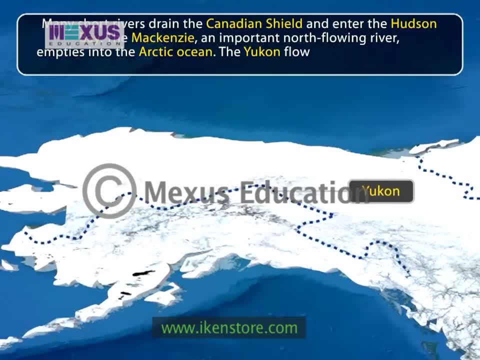 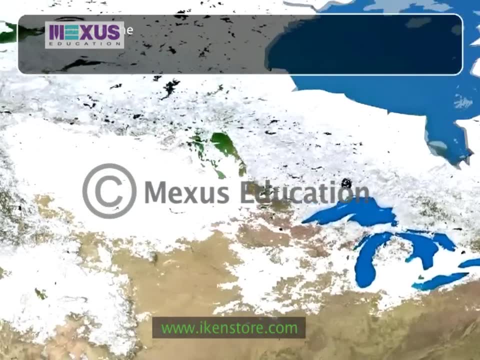 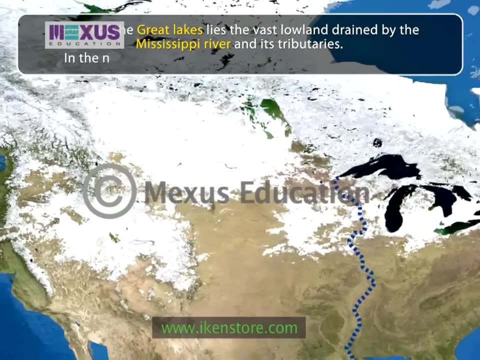 The Yukon flows through Canada and Alaska and empties into the Bering Sea. South of the Great Lakes lies the vast lowland drained by the Mississippi River and its tributaries. In the northern part, these lowlands are called the Prairies. 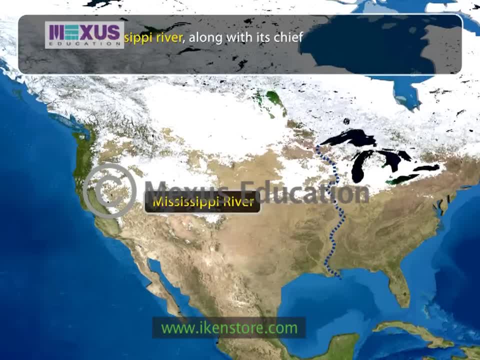 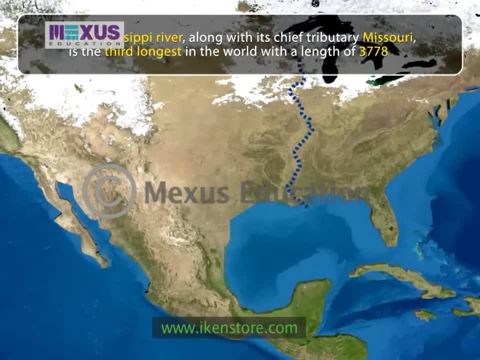 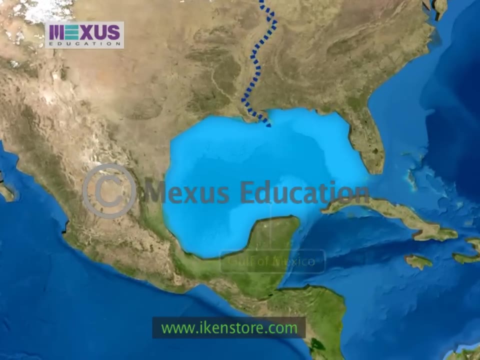 The Mississippi River, along with its chief tributary, Missouri, is the third-longest river in the world. With a length of 3,778 kilometers, it forms a large delta before flowing into the Gulf of Mexico. The Mississippi River is richly celebrated in American literature. 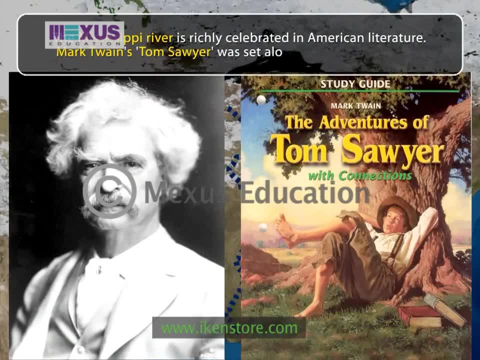 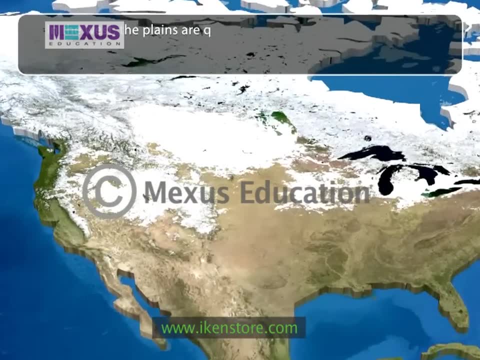 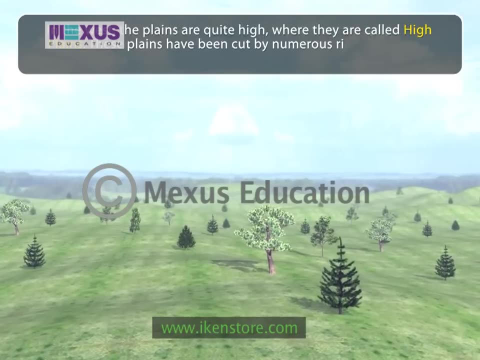 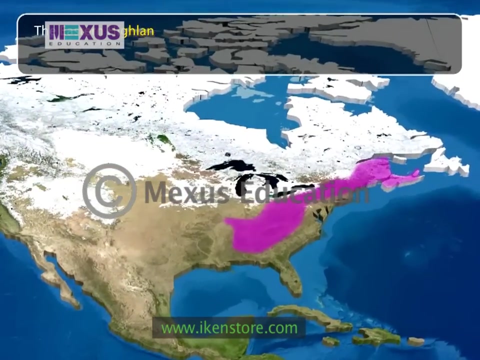 Mark Twain's Tom Sawyer was set along the Mississippi River. In the west the plains are quite high, where they are called High Plains. These plains have been cut by numerous rivers and many deep valleys can be found here. The Eastern Highlands, or the Appalachians, are a 2,575 kilometers long chain of mountains. 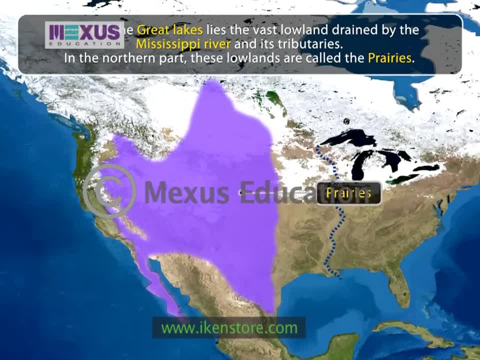 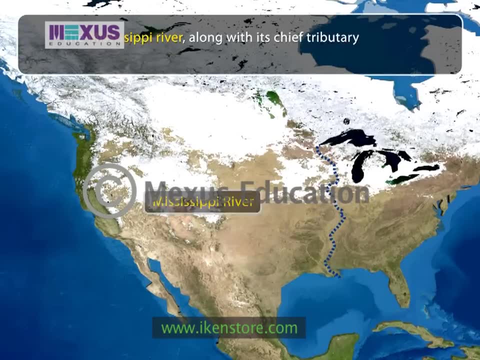 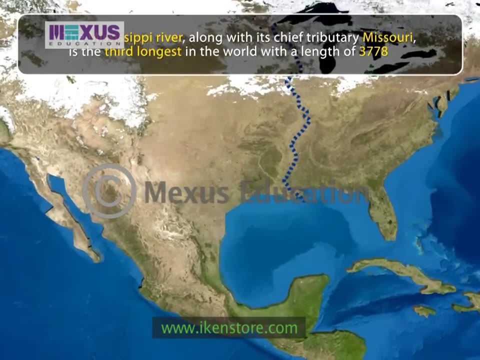 In the northern part. these lowlands are called the prairies. The Mississippi River, along with its chief tributary, Missouri, is the third longest river in the world. With a length of 3,778 kilometers, it forms a large delta before flowing into the Gulf of Mexico. 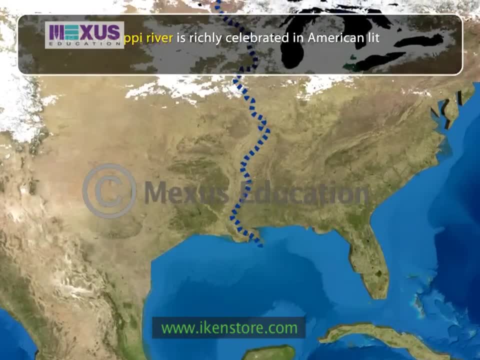 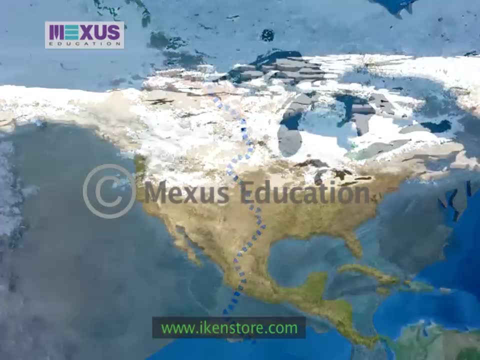 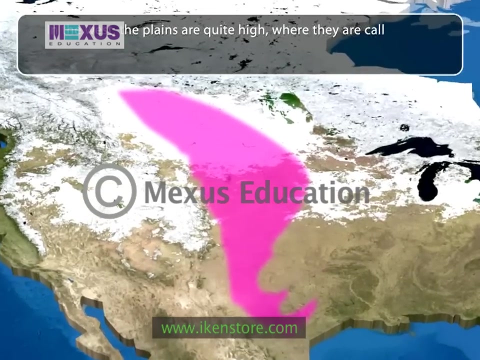 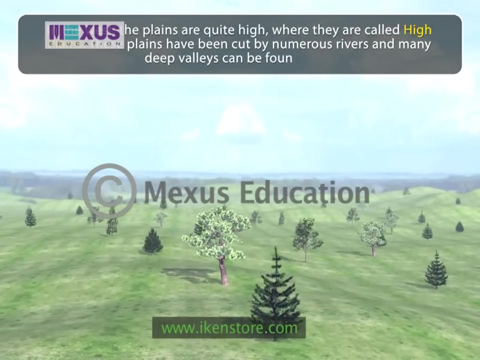 The Mississippi River is richly celebrated in American literature. Mark Twain's Tom Sawyer was set along the Mississippi River. In the west the plains are quite high, where they are called high plains. These plains have been cut by numerous rivers and many deep valleys can be found here. 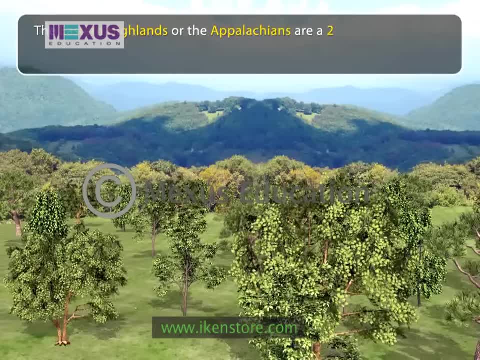 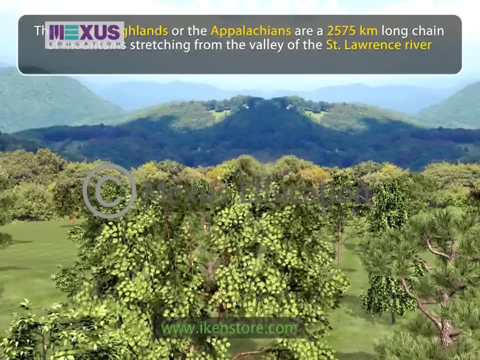 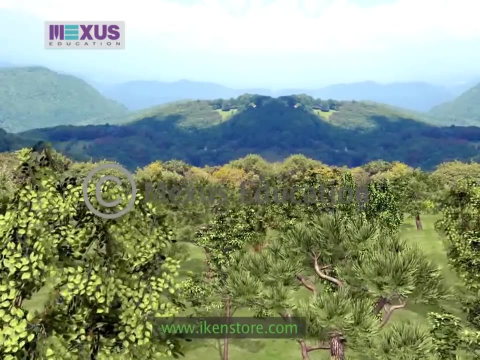 The Eastern Highlands, or the Appalachians, are a 2,575 kilometers long chain of mountains stretching from the valley of St Lawrence River down through most of eastern United States. They are not very high, being below 2,000 meters in most places. 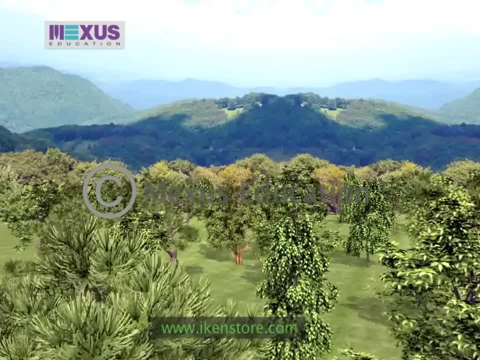 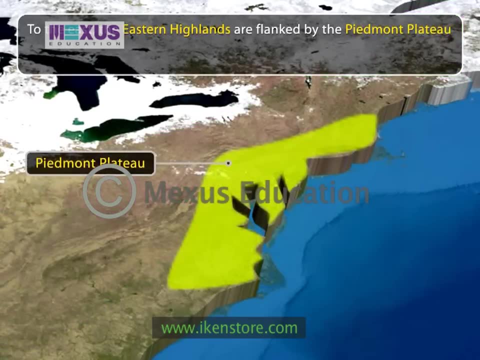 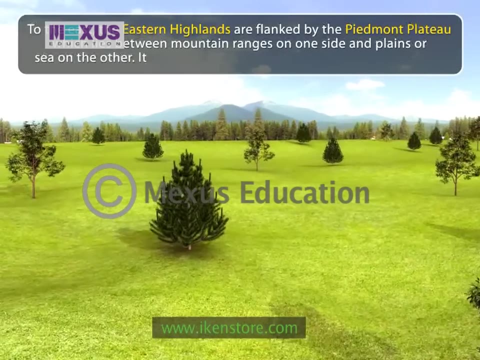 These are old-fold mountains and are made up of ancient rocks. To the east, the Eastern Highlands are flanked by the Piedmont Plateau, which lies between mountain ranges on one side and plains or sea on the other. It slopes steeply down to the Atlantic coastal plain. 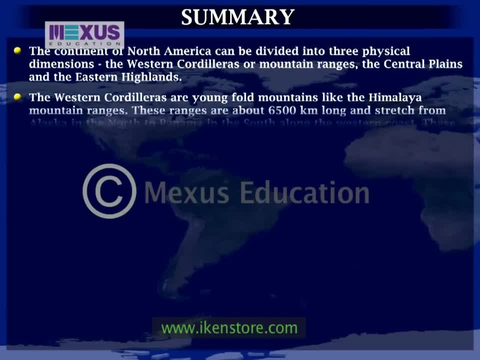 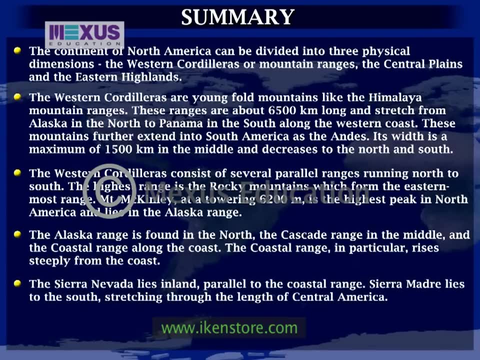 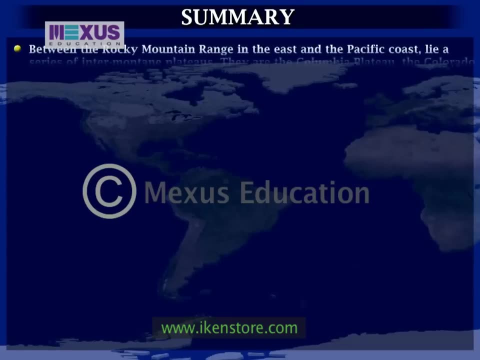 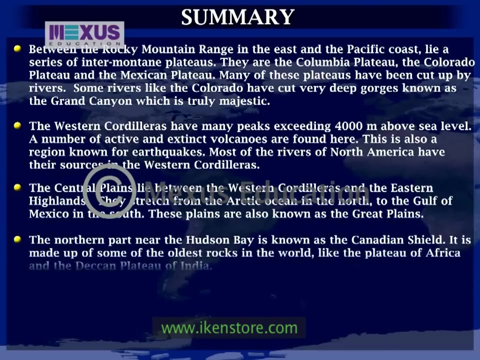 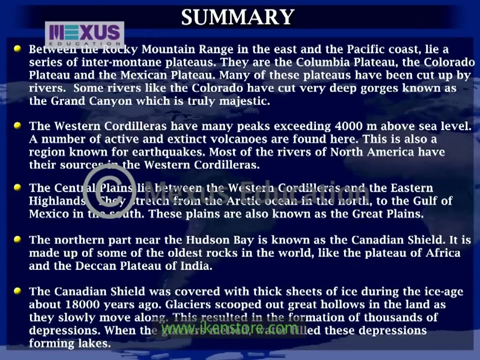 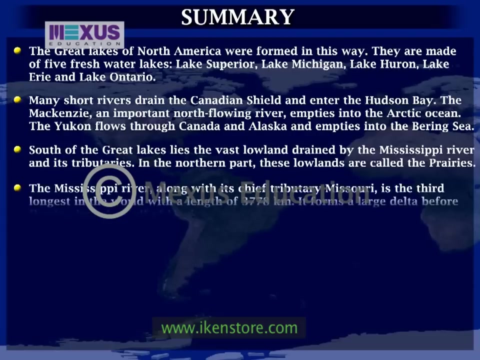 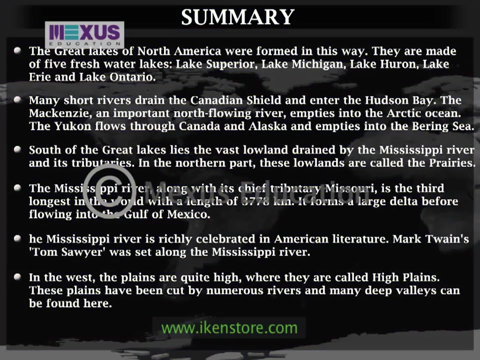 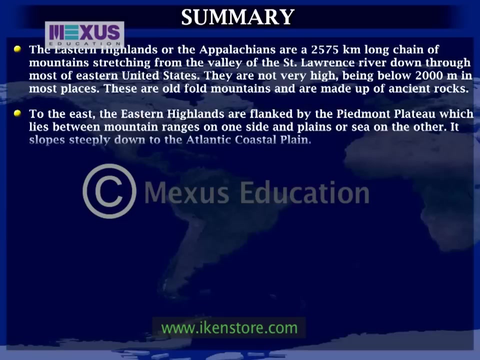 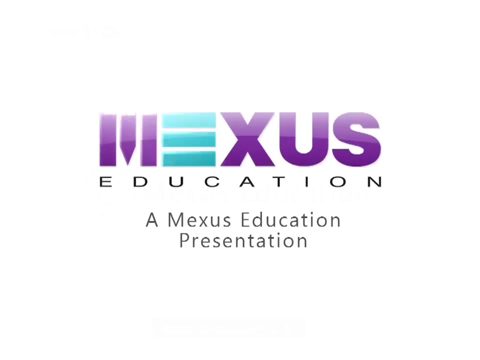 The Piedmont Plateau is surrounded by sandstone. © transcript Emily Beynon. © transcript Emily Beynon.